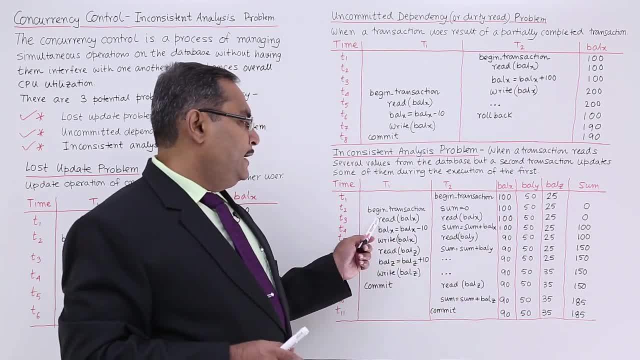 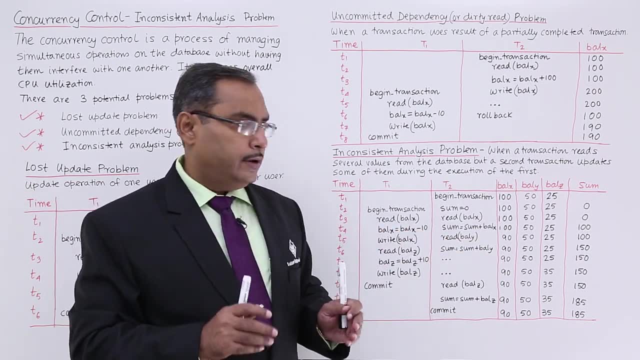 is equal to 0.. So sum is has got initialize with 0. read valence x: read valence x. valence x is having value 100.. So both the transactions have read 100.. Valence x is equal to valence. 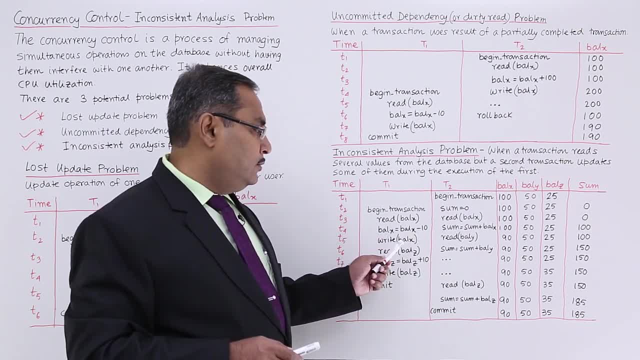 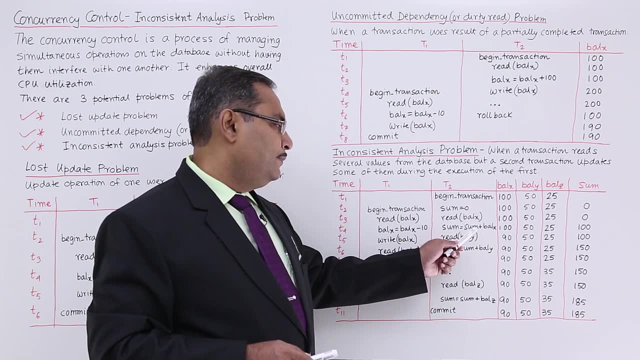 x minus 10.. So it has become 90.. But until you are writing this 1 on the data base, the value will still remain with 100.. This 100 is getting added to the sum, So sum has become. 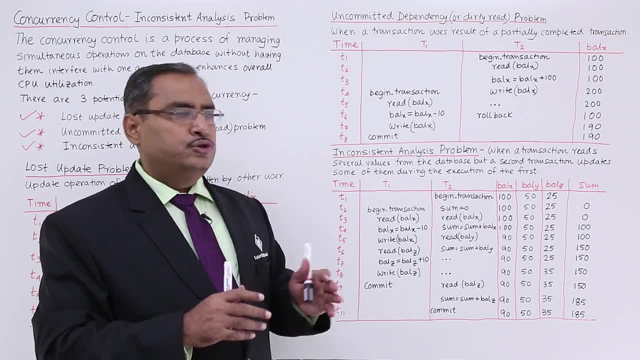 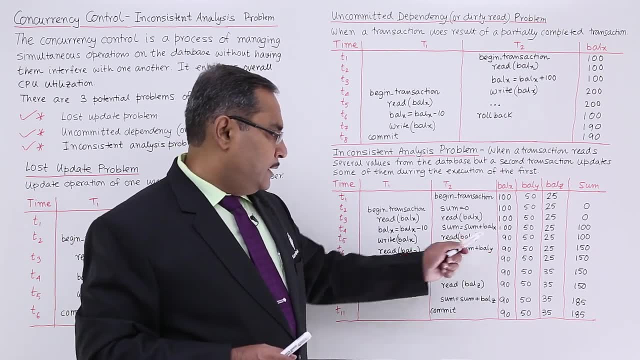 100.. So sum is a memory variable. So that is why the sum is getting added. sum has become 100.. Now write balance x. So the balance x has become 90 and rest of the cases. I am not dealing with the balance x, So 90 will be maintained. Now it is reading. 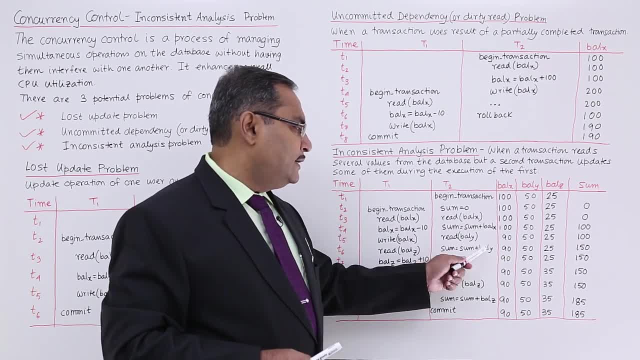 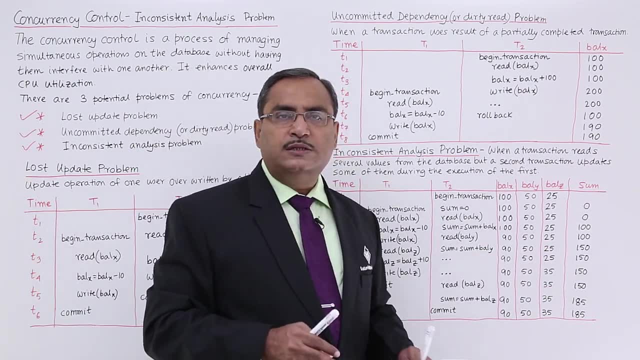 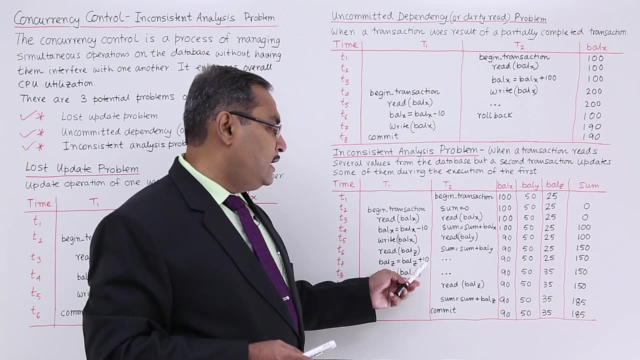 balance y, So balance y is 50 and sum is equal to sum plus balance y, So 50 will get added with the sum. Sum was having the previous value 100. So the sum value has become 150.. In the meantime it has read balance z and balance z value has got incremented by 10.. 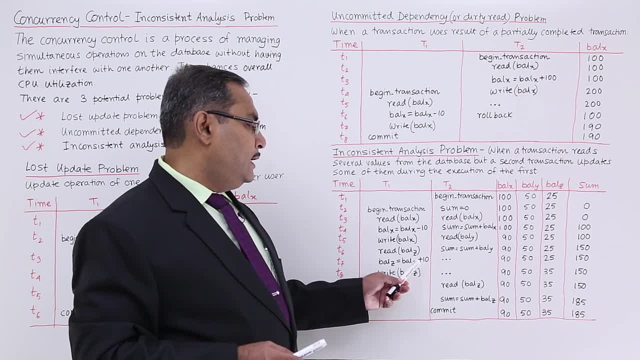 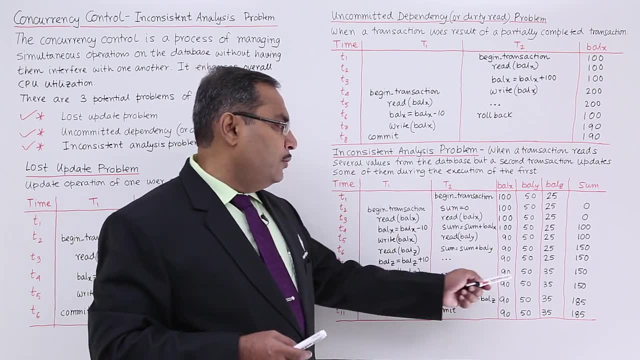 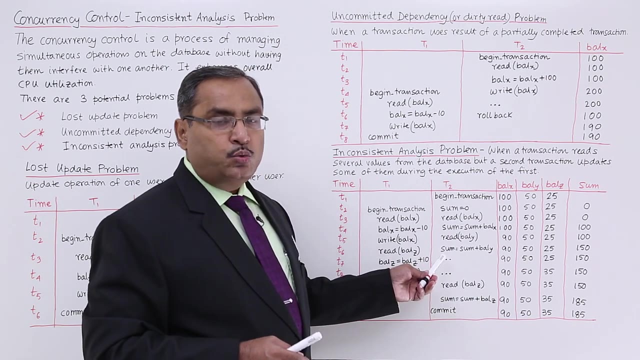 So initially balance z value was 25.. So it has got incremented by 10. So it is still with 25 because it has not been written on to the database. So write balance z. Now it has become 35 for the rest cases Now here, after doing the sum of balance y with: 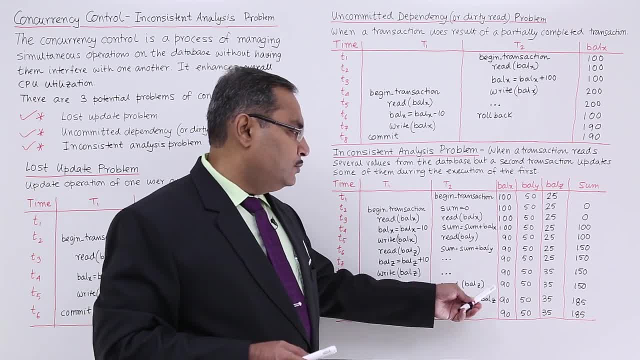 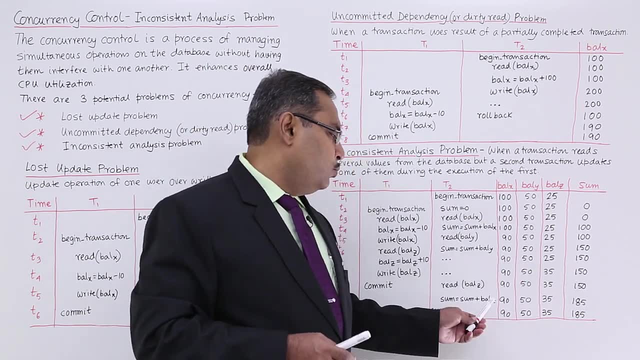 the variable sum. now it is reading the balance z value. Now the balance z value has got updated, So now it is 35. So sum value was 150, with the 35 is getting added, So it is becoming. 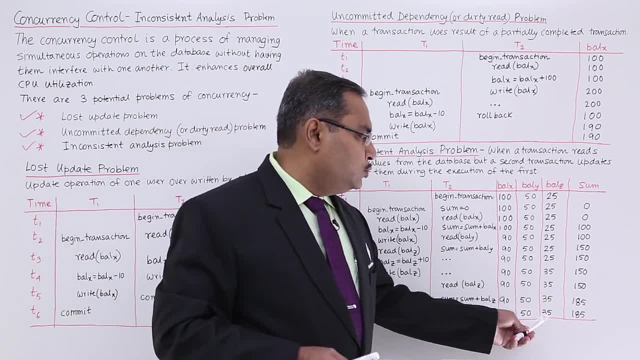 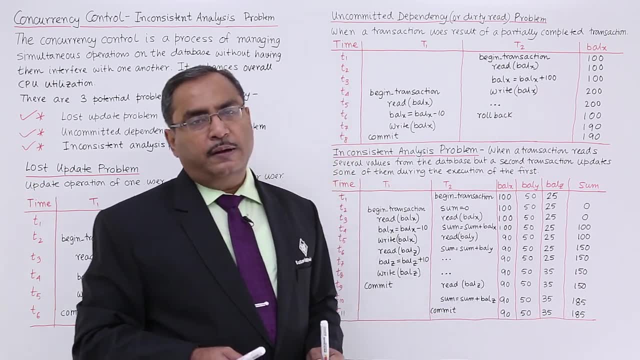 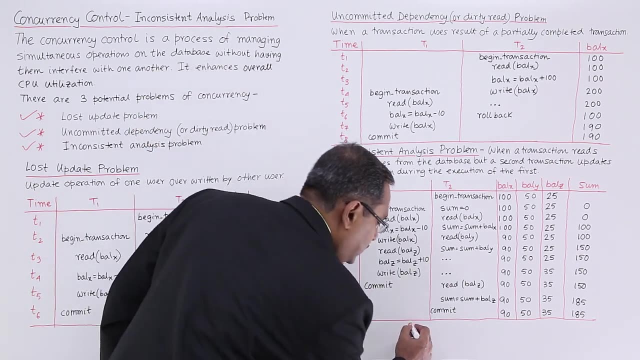 185. And in this way, last values, updated values for balance x, balance y and balance z, and sum are 90,, 50,, 35 and 185 respectively. So that is the issue. Now, what is the problem? Problem here is that, here you see, this 185 has been obtained. 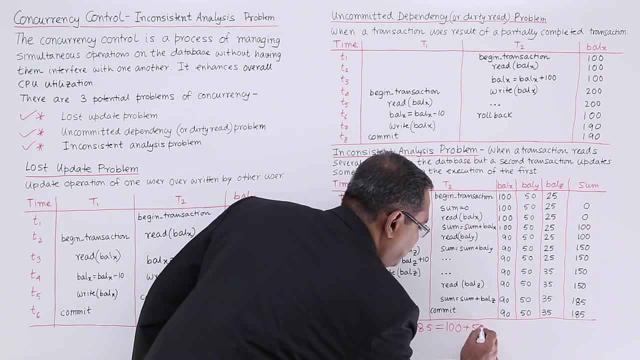 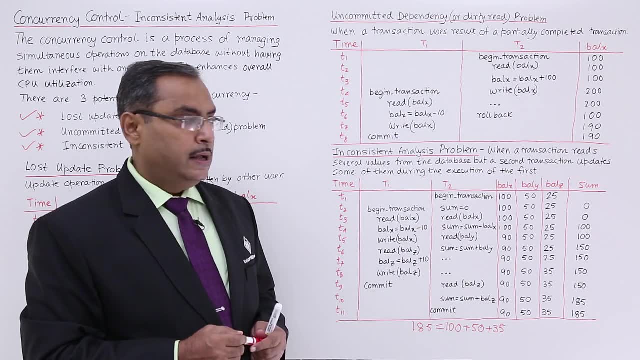 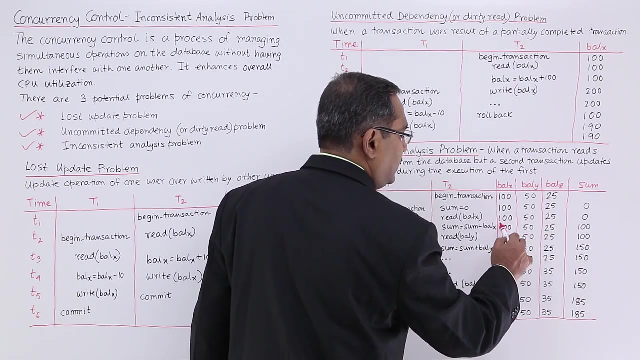 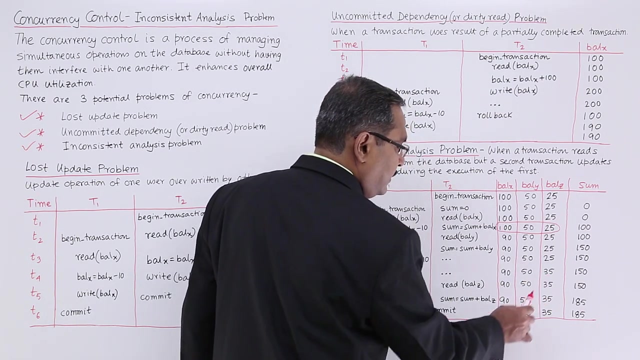 by adding 100.. 150 and 35. Since 185 has been obtained from 100,, 50 and 35. Now you see, when the value of balance x was 100,, then the balance z was 25.. It take any instance. but when the balance z has become 35, because I require 35 here- 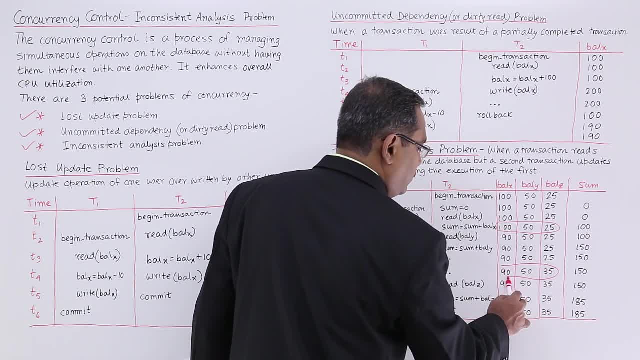 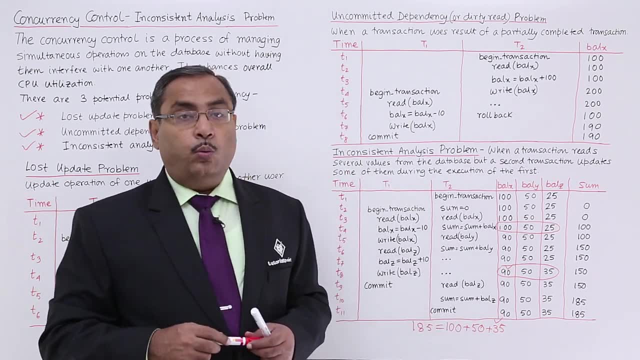 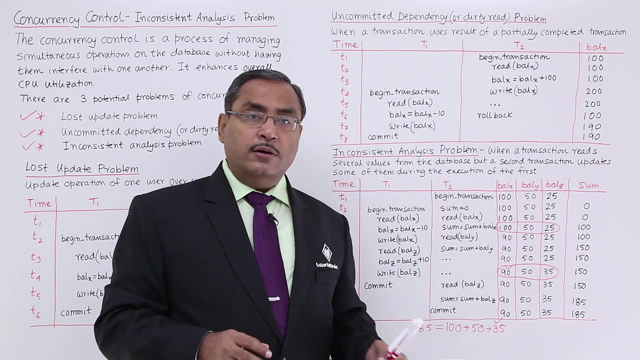 So when the balance z has become 35, then balance x has become 90. So this curve is combination, that is, 150 and 35 was not found in any one of the any one of the instances of the database, So that means this sum has been made of the values obtained from. 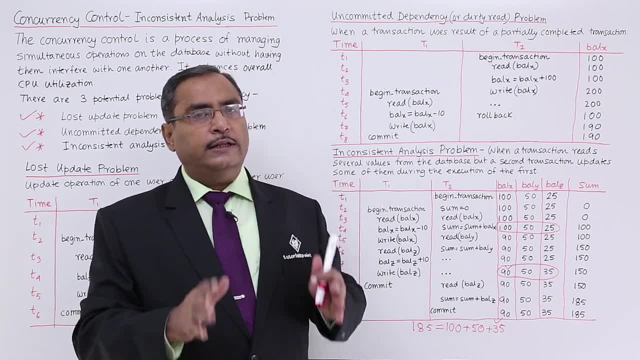 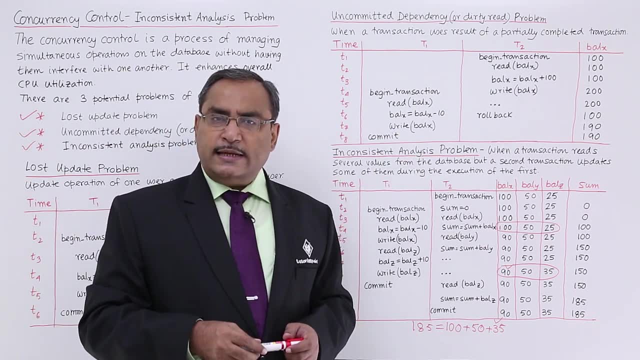 the database at different instant of time, not in the same instant. So that is known as the inconsistent analysis problem. So we know that instance of a database means, at any instant of time, the content of the database. So these values are available in. 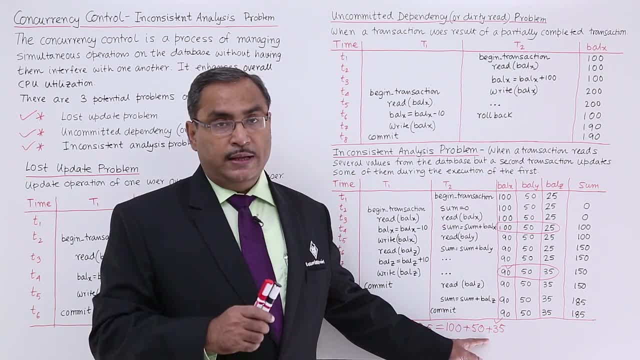 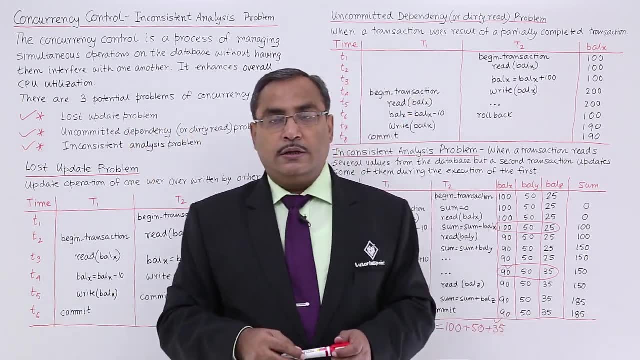 different instance of the database, not in the same instance. So that is a problem that is known as inconsistent analysis problem. So there are three problems are there? Now, in the next videos we will be going to discuss what are the different remedies, what are? 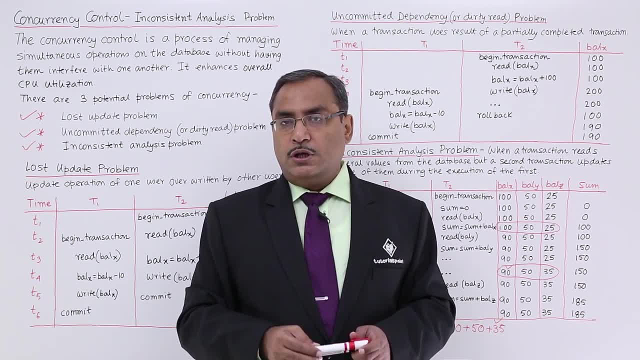 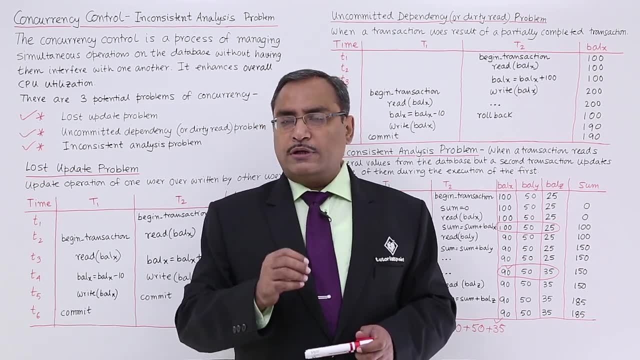 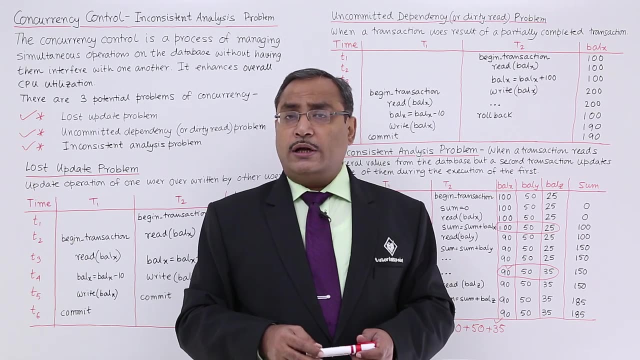 the different solutions for all these three problems. So we will be having the solution. like your locking problem, We will be going for two phase locking. One of the solution will be your time stamping and another solution will be your optimistic scheduling. So there will be three solutions We will be discussing. 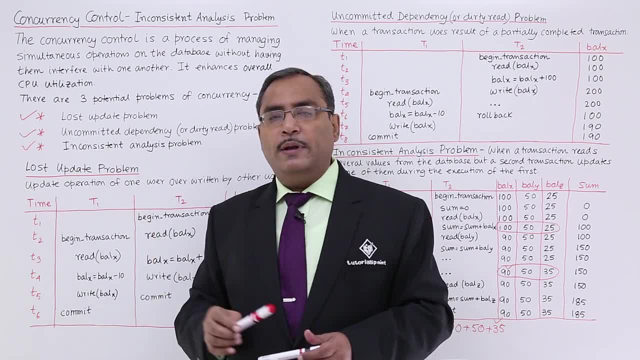 all these three solutions and other solutions of these problems in the next videos. Please watch all of them to have a knowledge on this transaction management. Thank you, 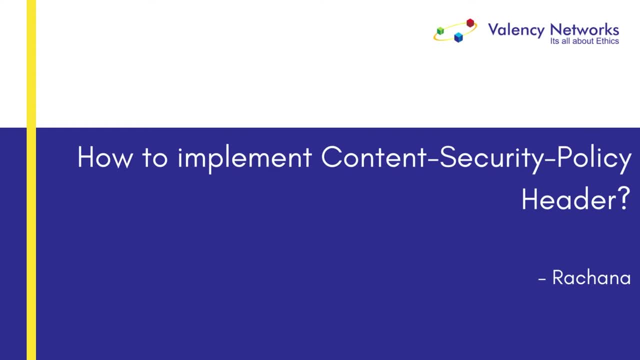 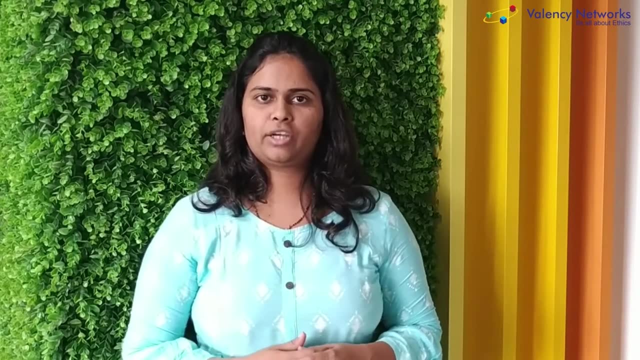 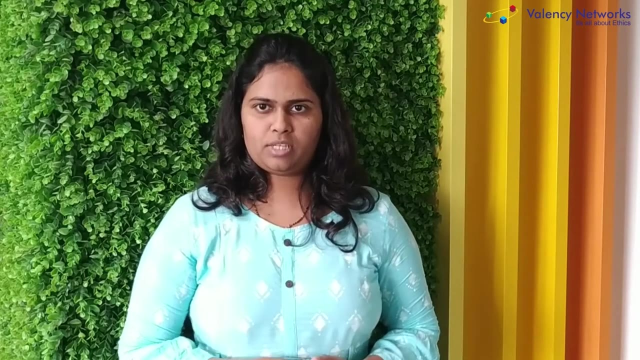 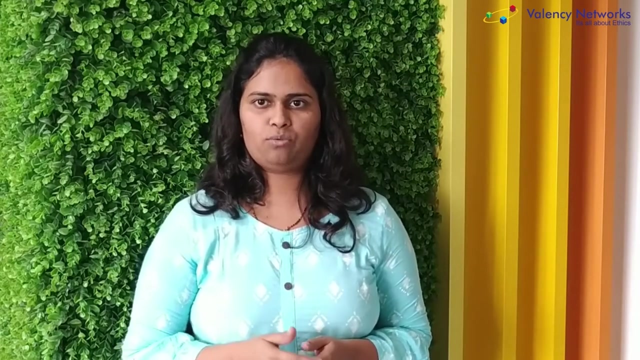 Hello everyone, today we are going to discuss about how to implement content security policy. Content security policy- that is, CSP. it uses to restrict what content loads onto your website. Using CSP, it adds a layer of protection to your website by stating rules of what is allowed and what is not allowed. 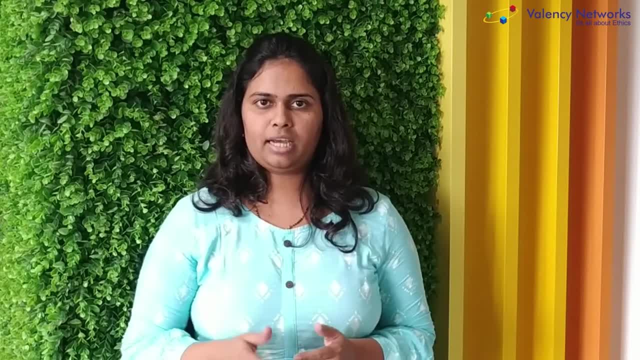 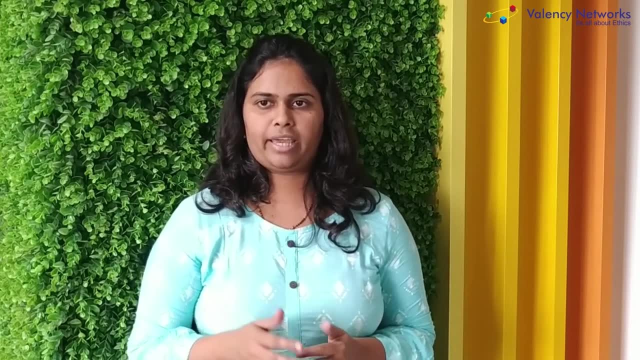 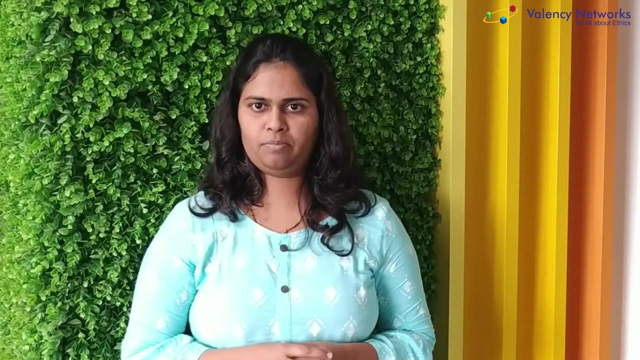 This is very helpful to defend against the attacks such as content injection and exorcist. Now, to implement this CSP, you must define list of allowed origins for all of the types of resources that your site utilizes. Also, it is very important to always define default SRC.